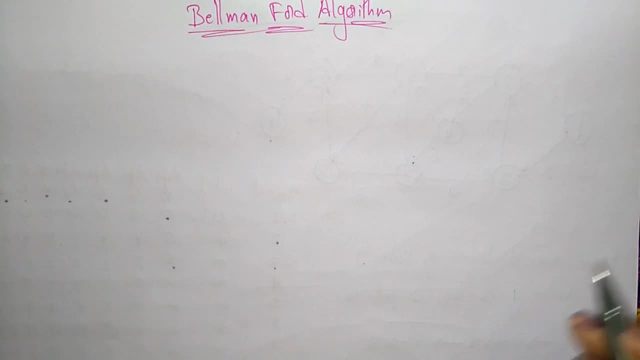 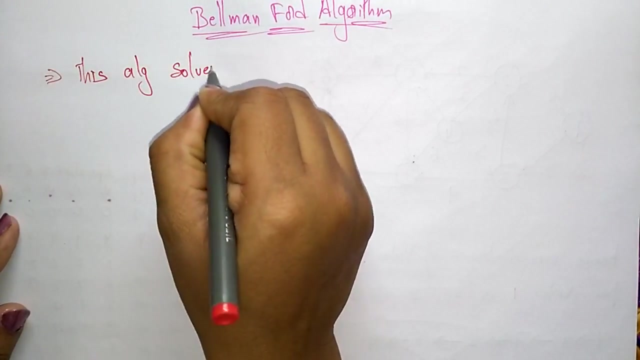 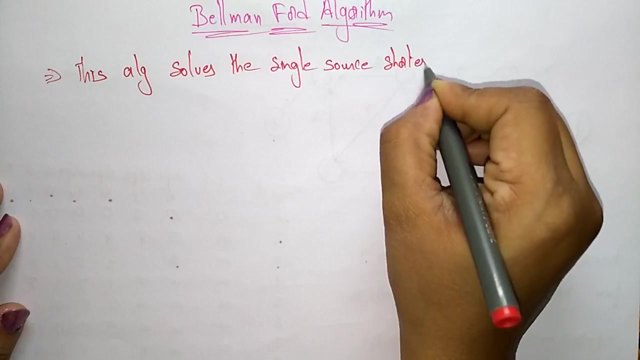 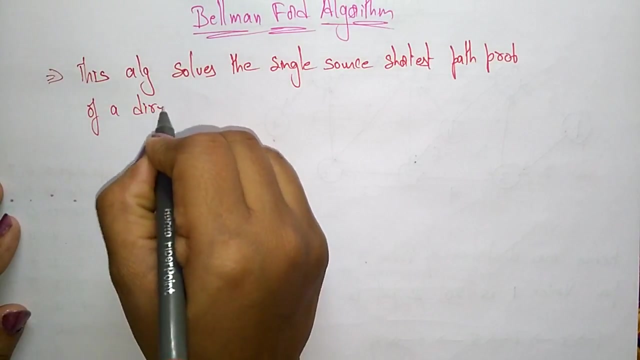 video I explained about the Dijikstra algorithm. Now let us see the Bellman-Ford algorithm. So actually this algorithm also solves the single source shortest path problem of directed graph. So this is a directed graph, whereas here Dijikstra is also a directed graph, but 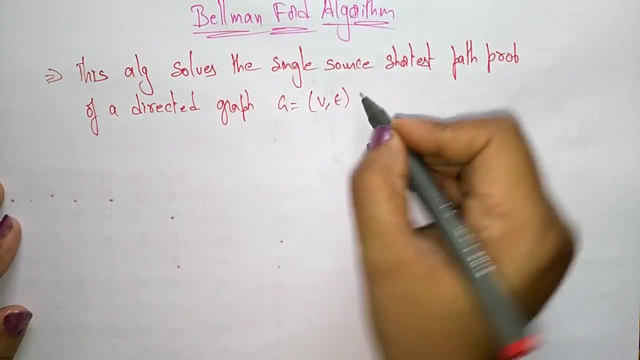 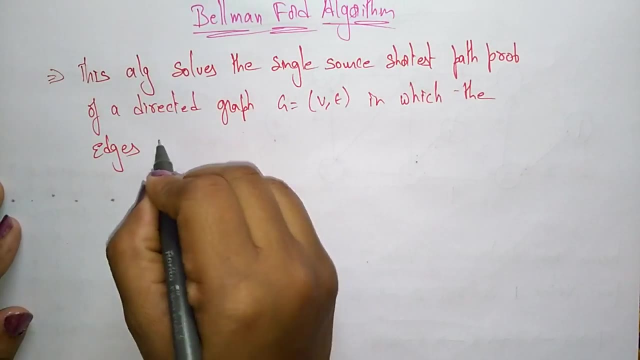 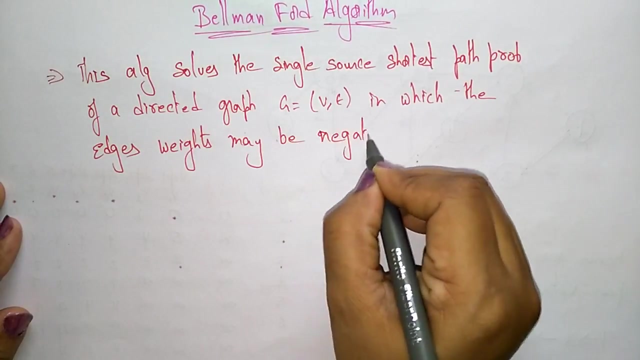 the only difference here is G, is V, E, So here Dijikstra, in which the edges weight. So whatever the weight that edges is having, those weights may be negative. So in Bellman-Ford you can, this can- accept the negative weights, whereas in Dijikstra 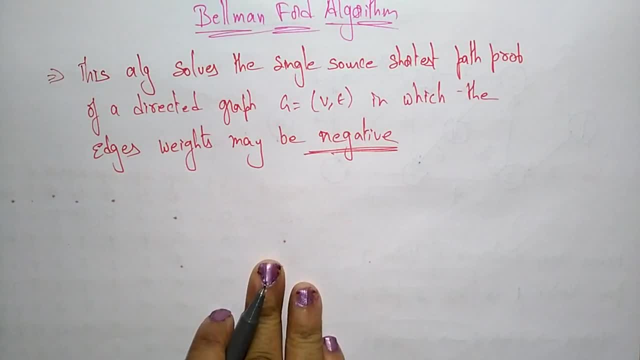 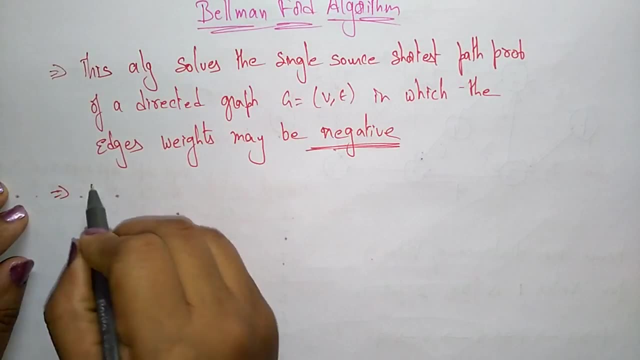 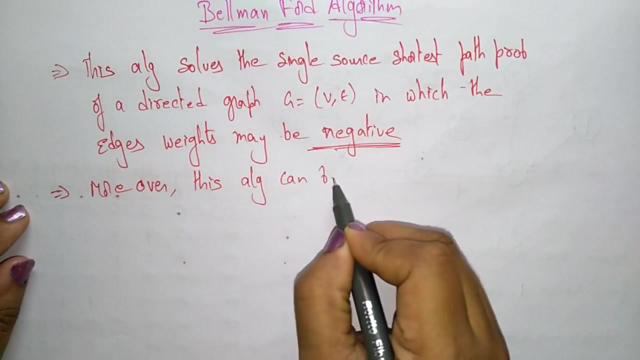 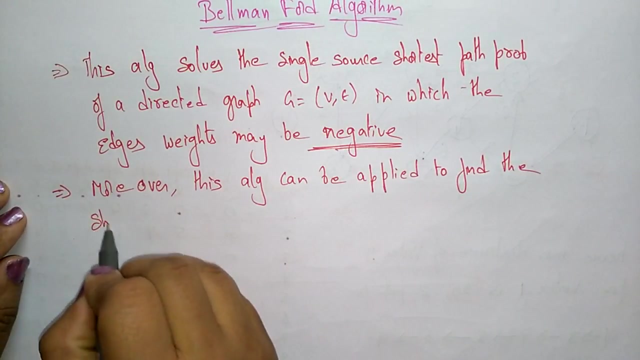 algorithm, only the non-negative weight should be accepted by the edges. But in Bellman-Ford you can take the negative values also, But, moreover, if you are taking the negative, moreover, this algorithm can be applied to find the shortest path. Shortest path if there does not? 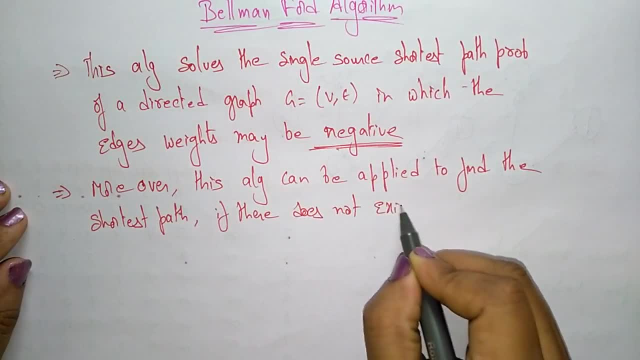 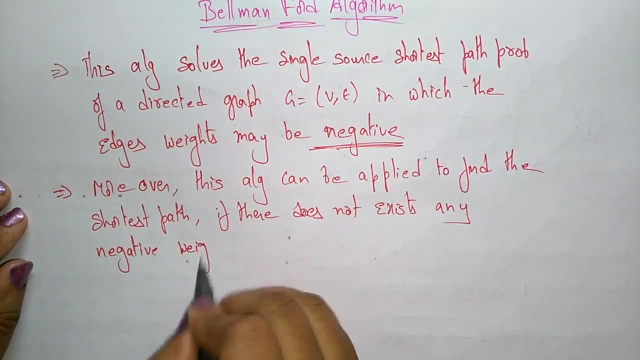 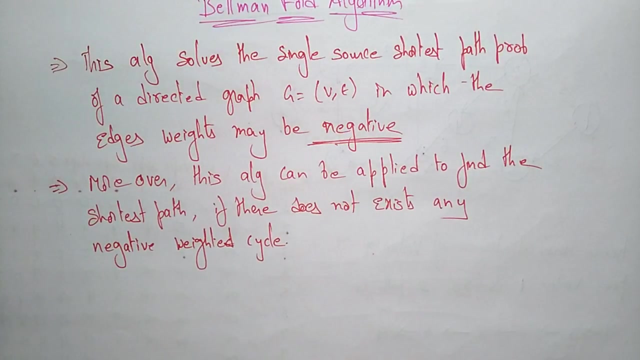 exist, does not exist any negative weighted cycle, any negative weighted cycle. So it can also be considered that it can take the non negative values also, and it does not exist that negative weighted cycles, Negative values, can be accepted, but negative weighted cycle cannot be accepted in Bellman-Ford algorithm. 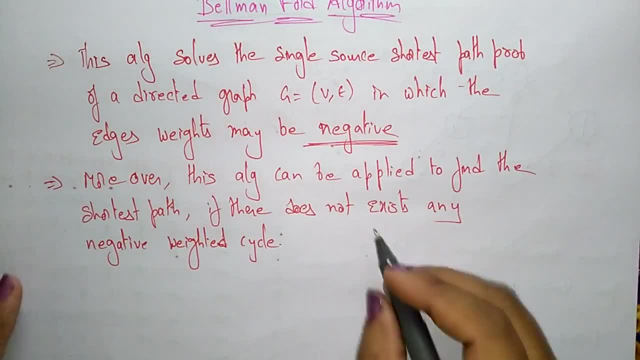 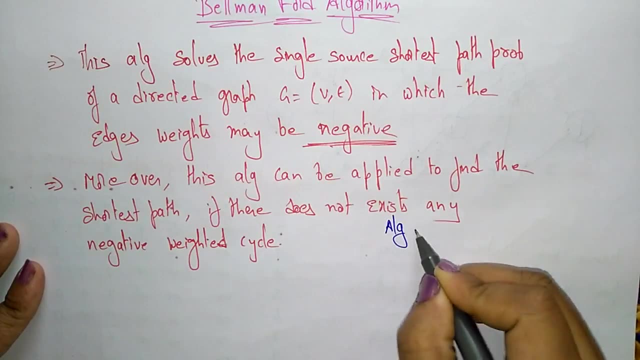 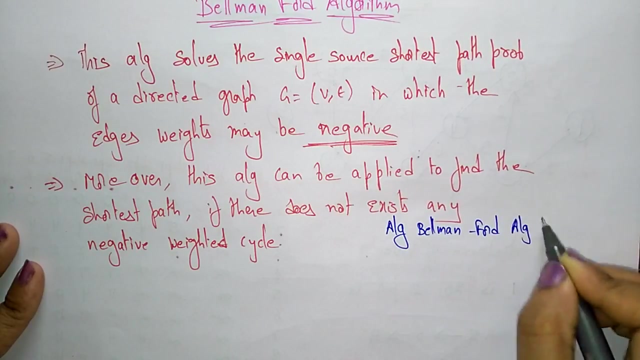 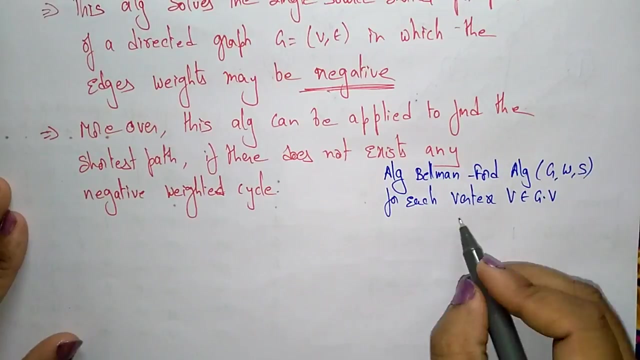 So let me write the algorithm for this Bellman-Ford. Here I am writing algorithm Bellman-Ford four. algorithm g, w, s. so just like for each, s is a starting vertex, g is the graph and w is the weight. vertex v belongs to g dot v. so now check v dot d. the destination should be infinity and v dot pi. 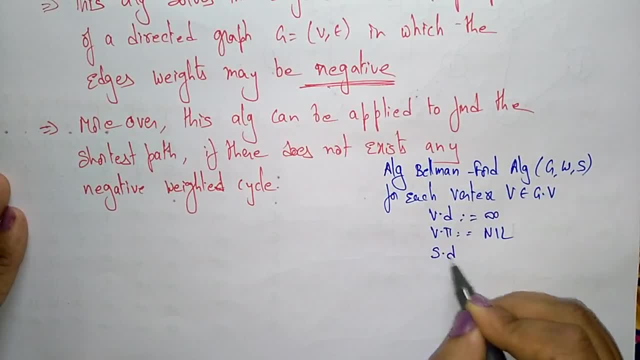 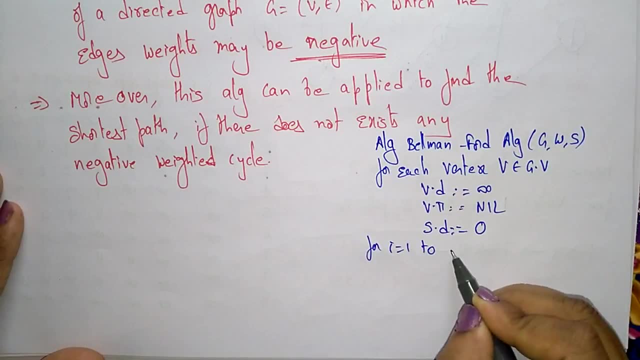 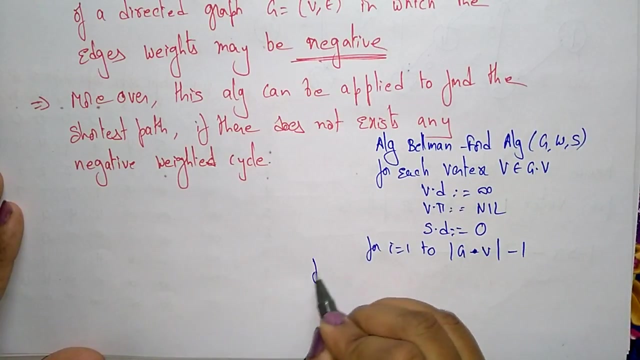 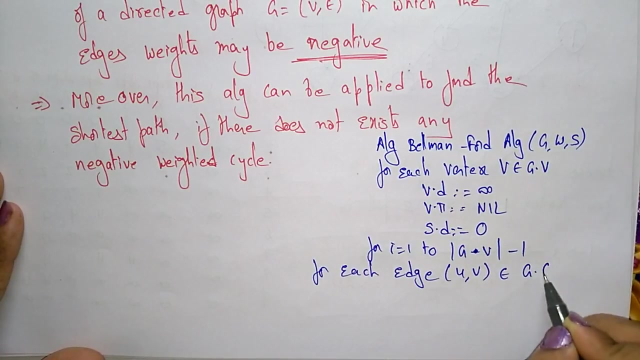 the starting should be make it as a nil and s dot d should be zero. start with a zero, for i is equal to one. two mod g, my g dot, sorry, g dot v minus one for each edge. u comma v belongs to graph dot, g dot, edges and condition: if: 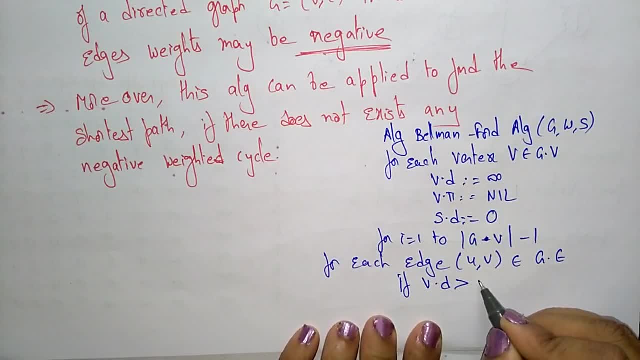 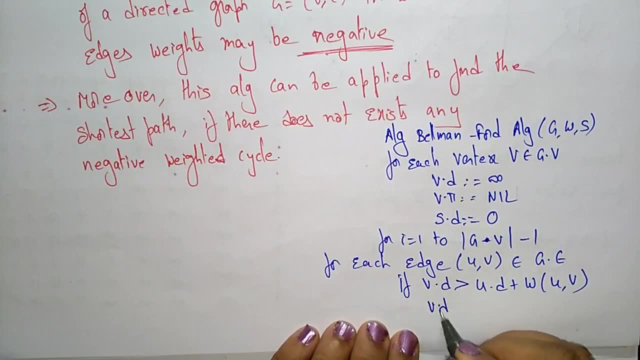 you v dot v same, just like well, uh, digester, v dot d is greater than u dot d plus w of u comma v v dot d, then you make it v dot d is equal to u dot d plus w of u comma v and v dot pi should be. 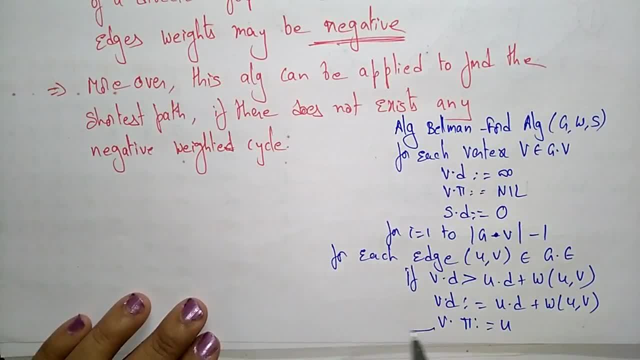 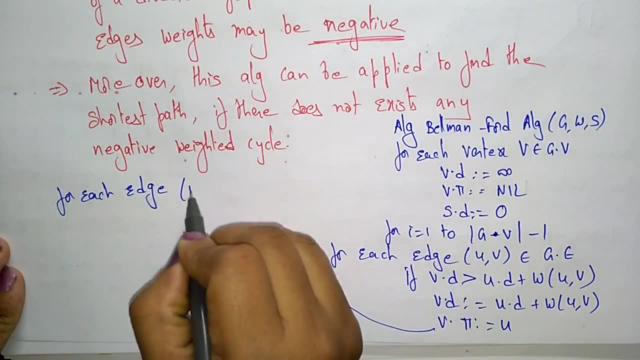 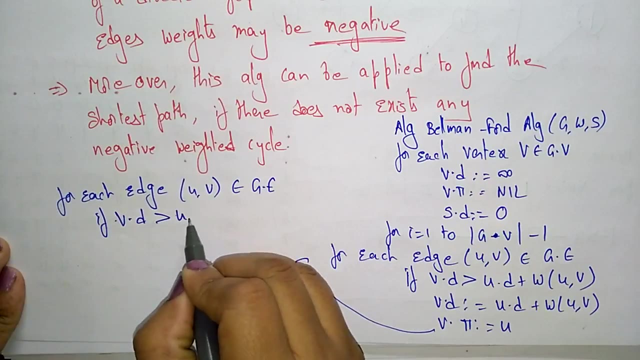 u. so up to here it is same for the digester algorithm. so after, after that, you have to check for each edge. u comma v belongs to g dot e if, if v dot d, v dot e is greater than u dot d u t r is greater than. 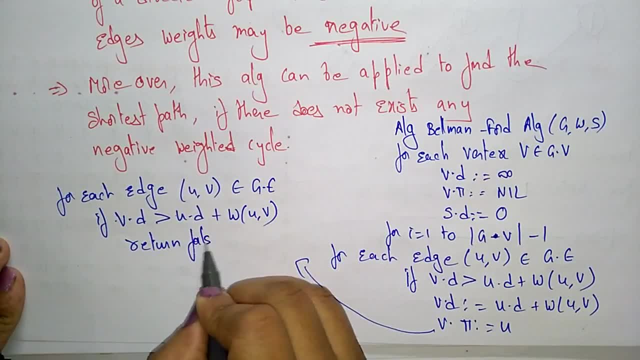 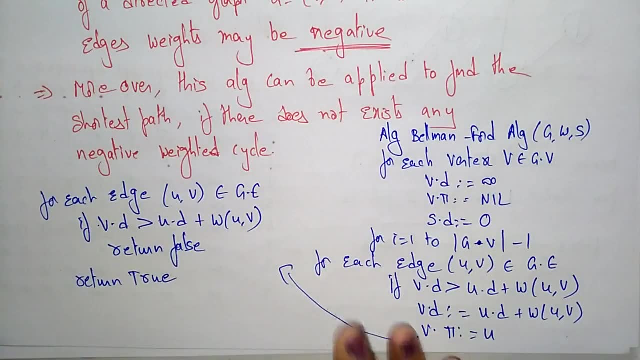 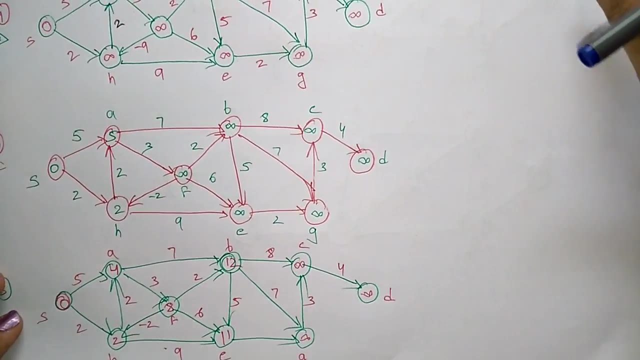 u dot t plus w of u comma v or w as 5 u u come a v belongs to g dot e, if v dot d, if so, to this absurdity, i mean if u was here. so here is an example for the bellman ford algorithm. so the starting this is the i have. 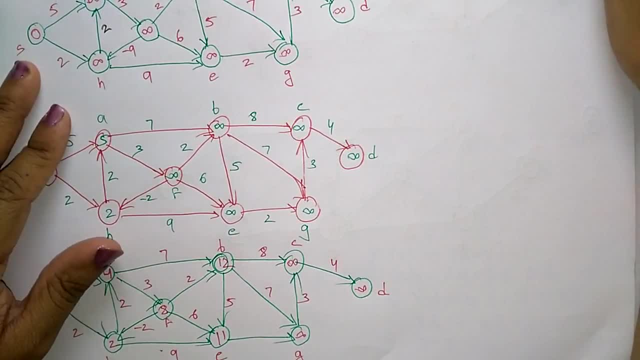 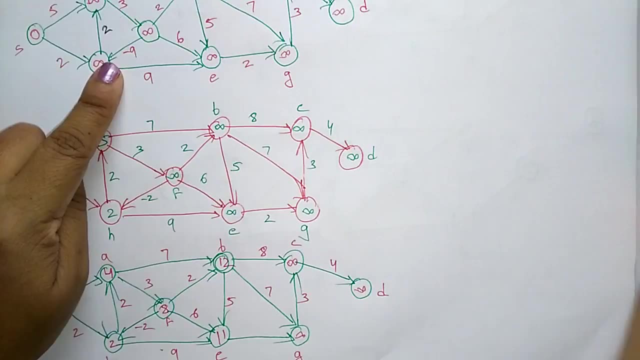 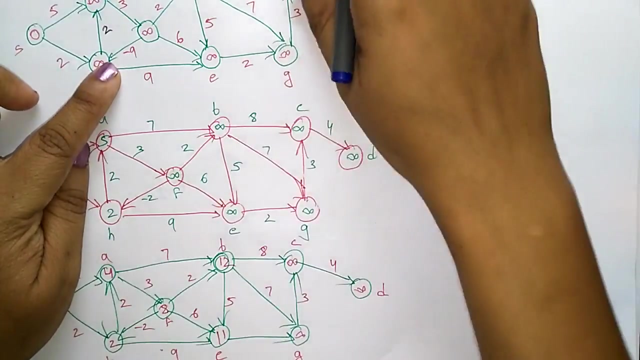 taken the graph, so this graph has negative edges also. you observe here: this is the negative edges also. this graph consisting of this graph has negative edges, but does not have any negative cycles. don't have. you don't have negative cycles, only negative edges are there, but it doesn't have. 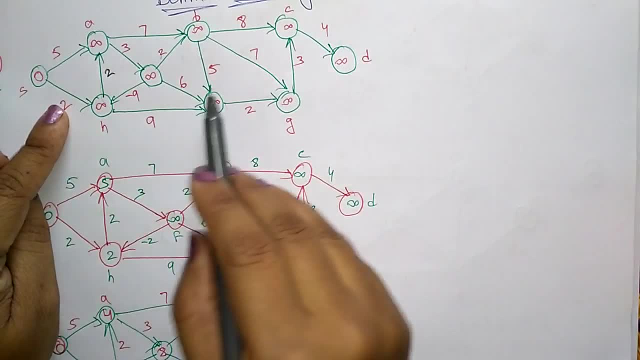 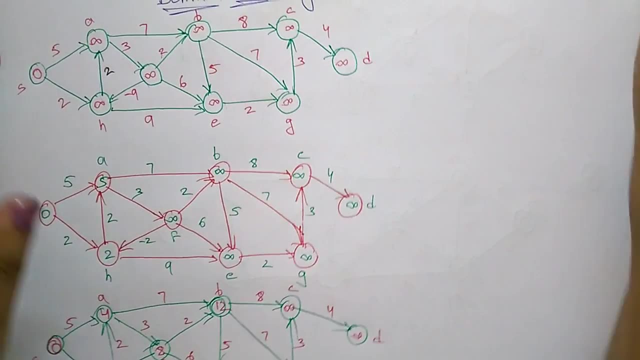 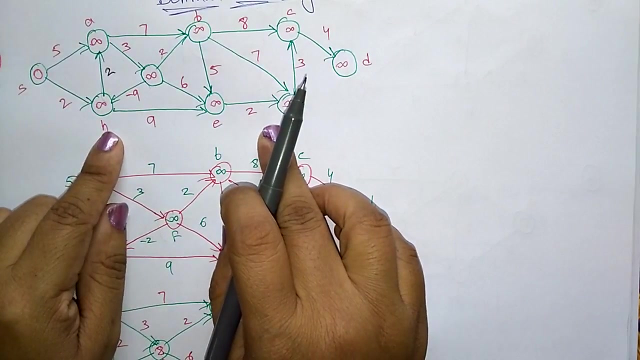 any negative cycles. so cycle means the complete connected graph, closed graph you call it so. hence the problem can be solved using this bellman ford. so this graph can helpful to solve the bellman ford algorithm. so first you have to check whatever the graph that they are given is ready to solve. 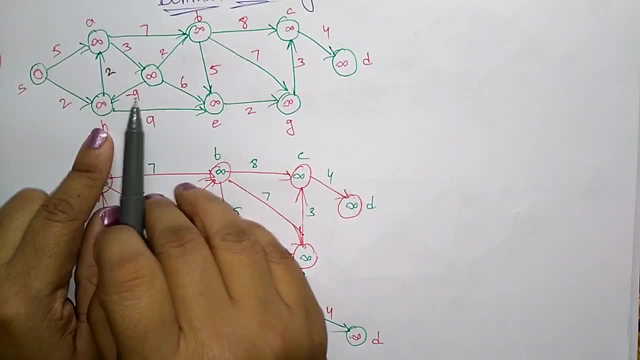 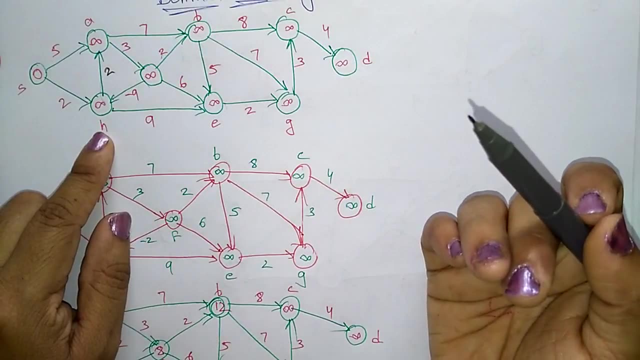 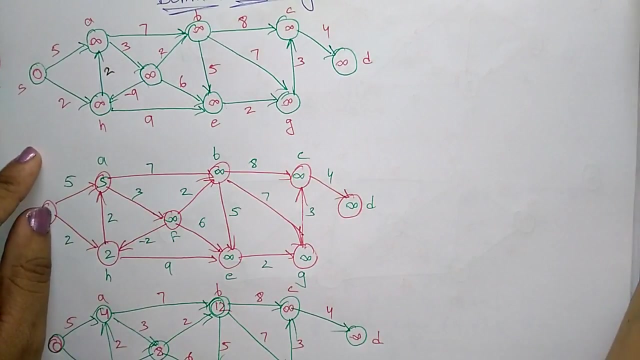 the bellman ford algorithm or not. so first see whether the negative values are there. if negative values are there, no problem, the bellman ford algorithm will solve the problem. all that, negative values also. but you have to consider there should not be negative cycles. so at the time of initialization all vertices except the source are marked by infinity. so here, 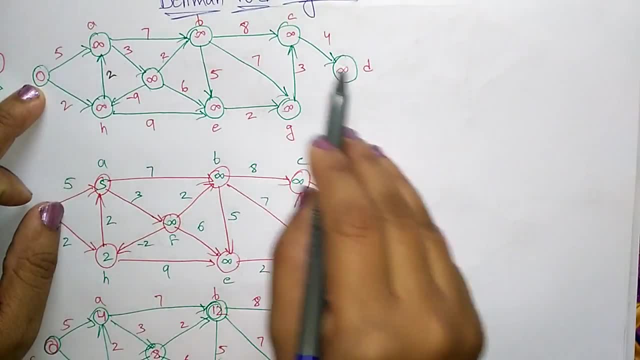 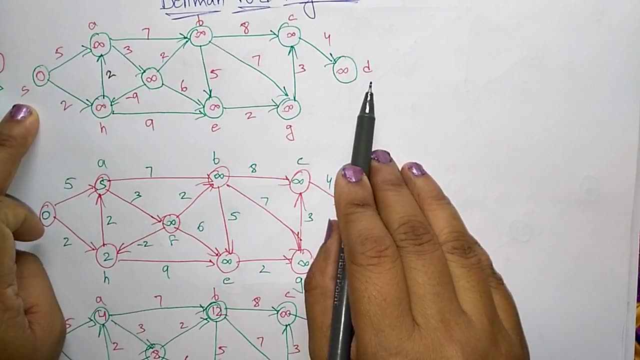 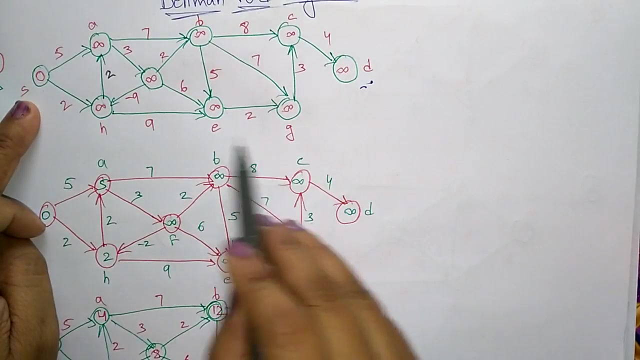 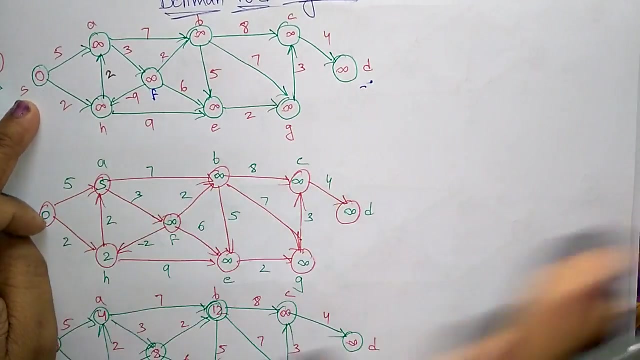 except the source. all the remaining vertices are marked infinity. okay, and this source should be marked as zero. this is the source and this is the destination. s is the source and d is the destination here. okay, here the vertices names: a, b, c, d, e, f. so this is the f, f, g, h. so these are the vertices and the. 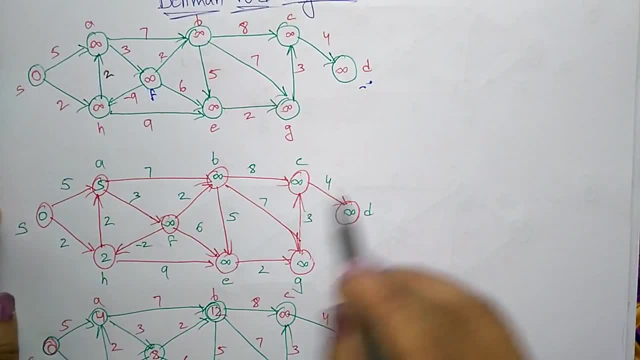 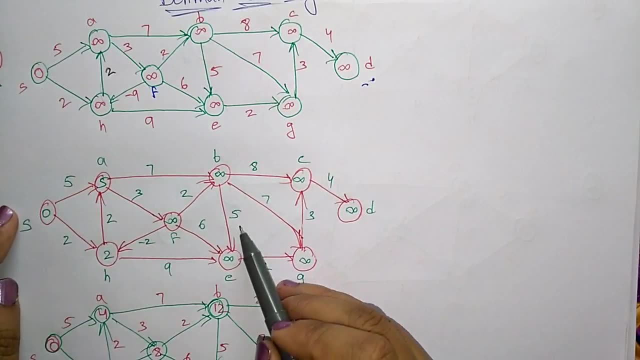 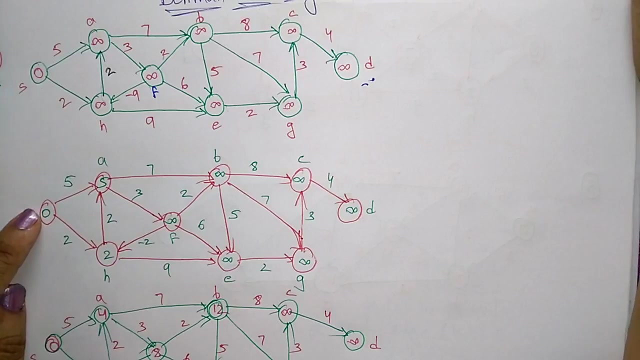 vertices, values, the weighted graph. so, coming to the first, in the first step: all the vertices, all the vertices. so, whatever the vertices, all the vertices which are reachable from source to destination, the source, or updated by minimum cost. so let me explain once again, in the first step. 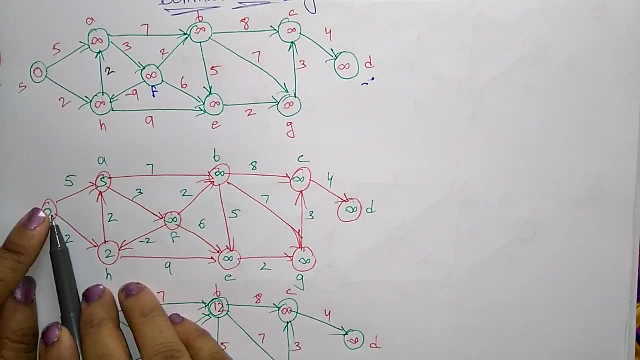 all the vertices which are reachable from. so this vertices is reachable from this vertex, source vertex, and this vertex is reachable from source vertex, so these two vertices are reachable. so that's why the vertices which are reachable from source vertex are updated by minimum cost. so you have to update it with minimum cost. hence a? n this, a and h are updated. with what values? 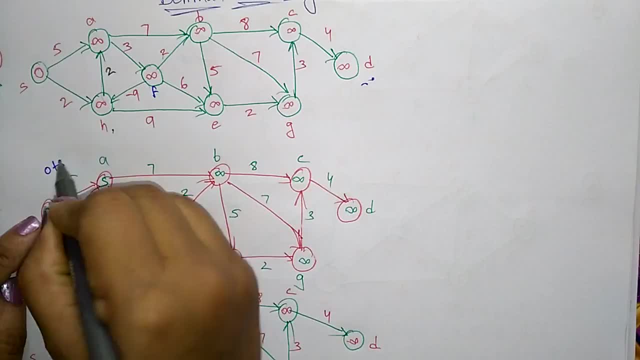 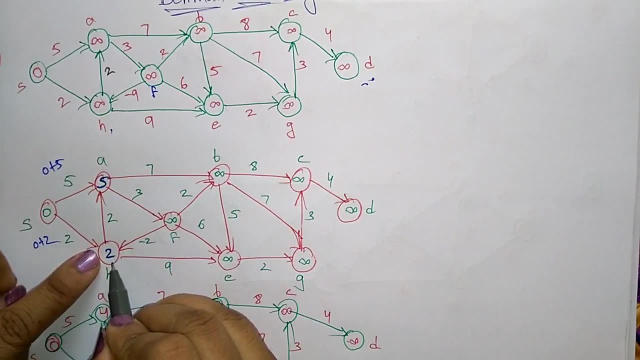 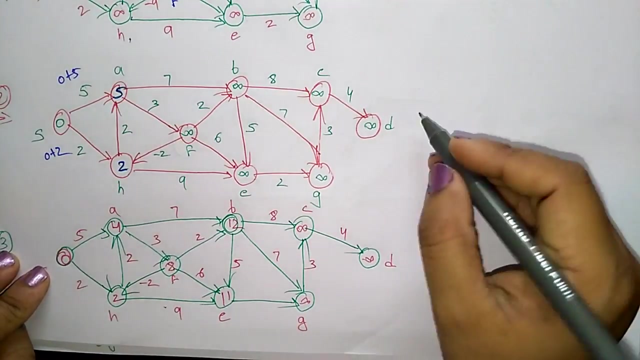 so 0 plus 5. okay, 0 plus 5, so the market has a 5 and this is 0 plus 2. i mark it as is 2, okay, so now coming to the next in the next step. so here in the next step, vertices a: 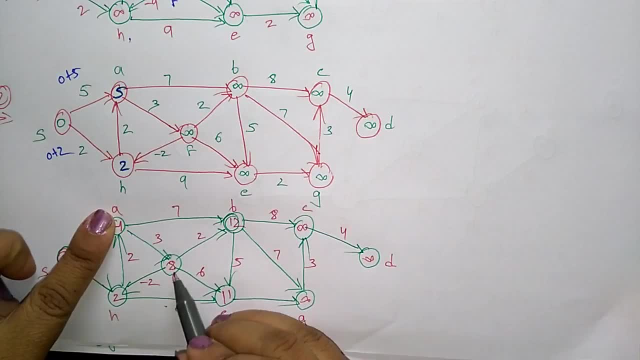 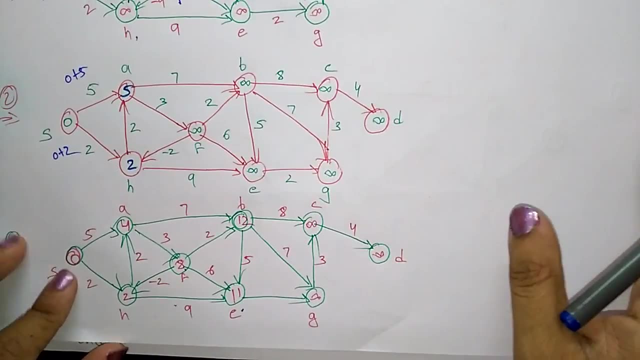 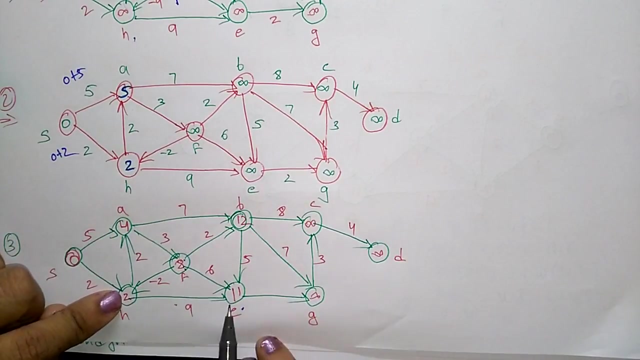 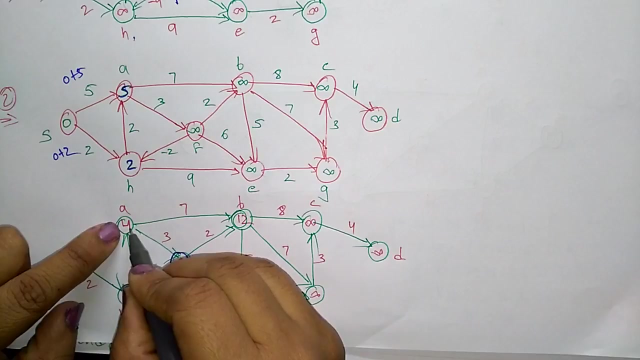 b, f, e. so already a, h is updated. next, the: the vertices that are reaching from the a or b, f, okay, and you have to take the e also because from h it reaching e. so all these three vertices. so from a, the reaching vertices, or from- this is a source. here- the reaching vertices are f and b and from. 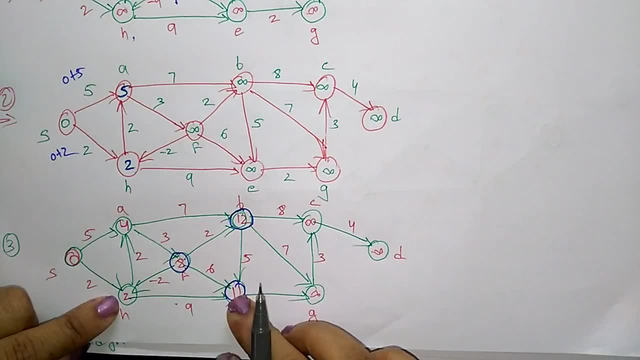 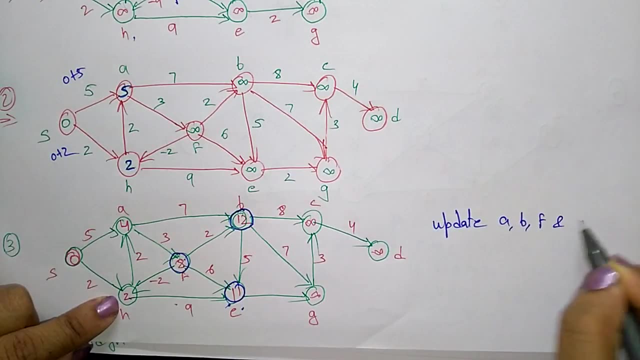 h the reaching vertices is from a to f and b, and from h the reaching vertices are f and b, and from is E. So this 3 has to be updated. So update A, B, F and E. So with what values we have? 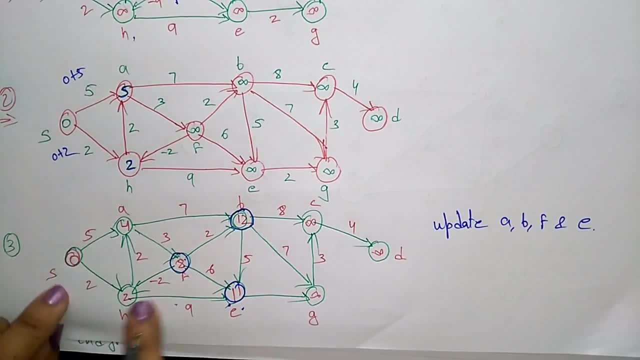 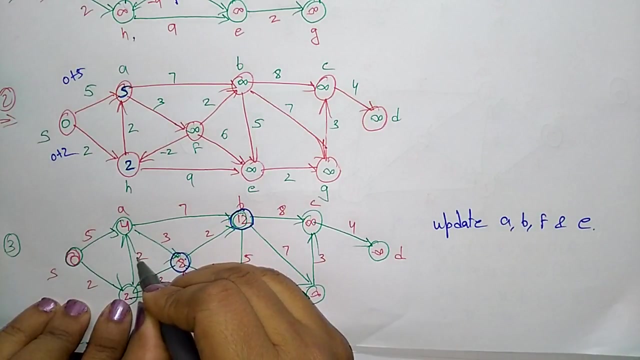 to be updated. So here the arrow is coming like this. So first you check this: 2.. So here the 2 is there and this is coming this side, So don't care this. So now check here: 2 plus 2.. Okay, 2 plus 2 becomes 4.. So, but here this is 5.. So just overwrite that and 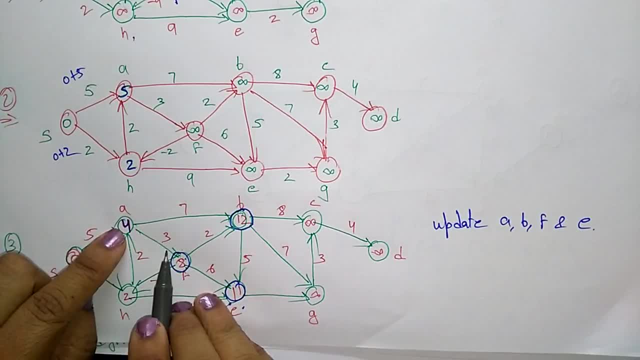 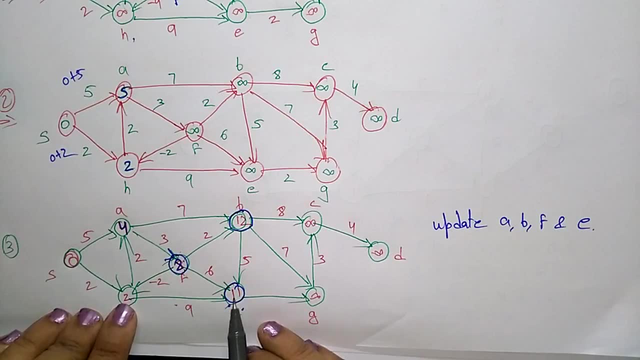 mark it as a 4 and add 4 plus 3. You will get 8.. The arrow is coming here, So 8.. And now check. So E. E has to be updated with what value? 2 plus 9.. 2 plus 9 is equal to. 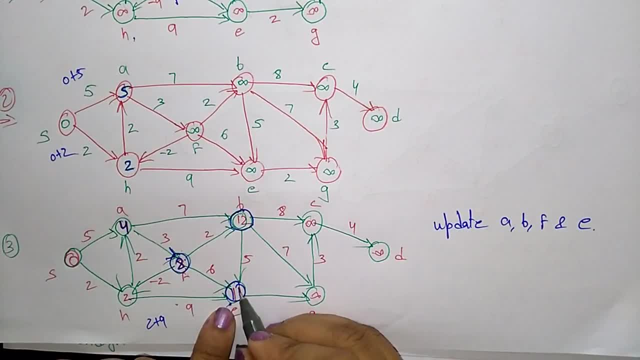 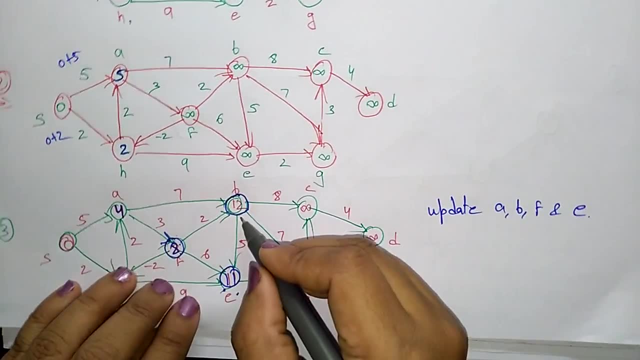 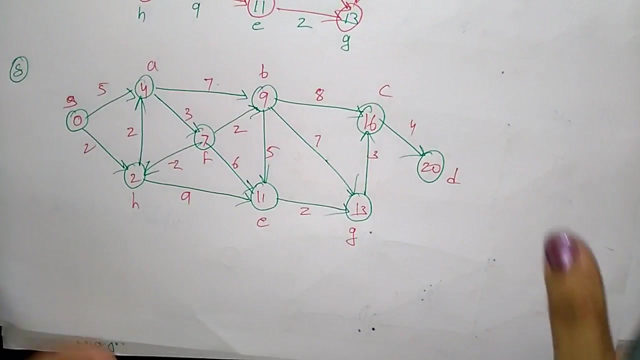 11. Okay, This is satisfied. Okay, And here E E has to be updated with what value? 2 plus 9.. Check, So this arrow is coming from like this. So up to here we updated. Now coming to the next step. So in the next step, following the same logic in the steps, what is this? 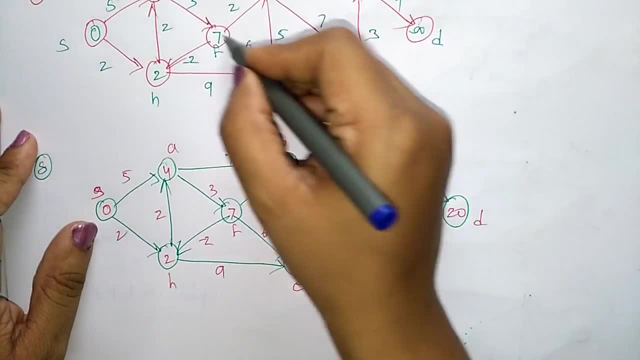 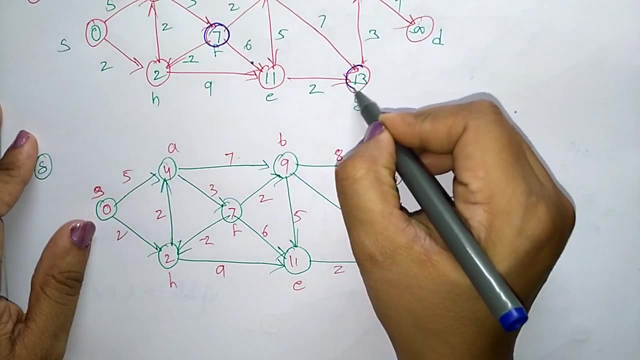 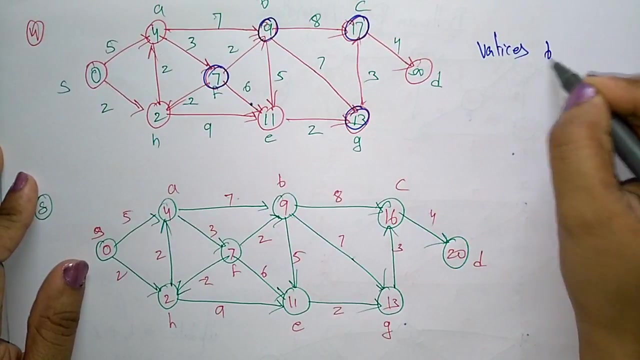 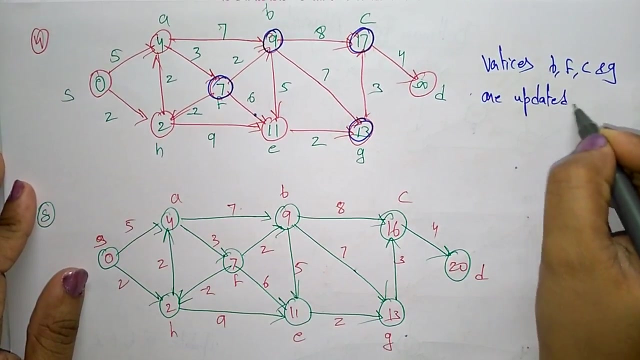 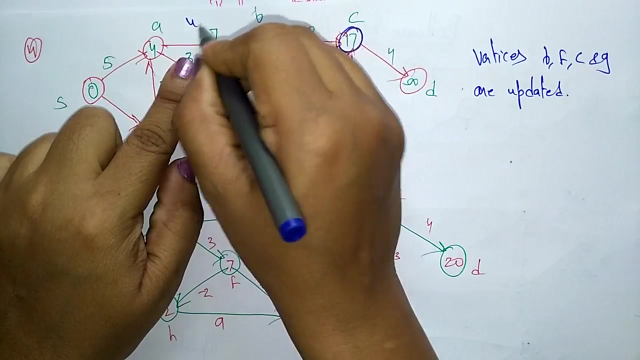 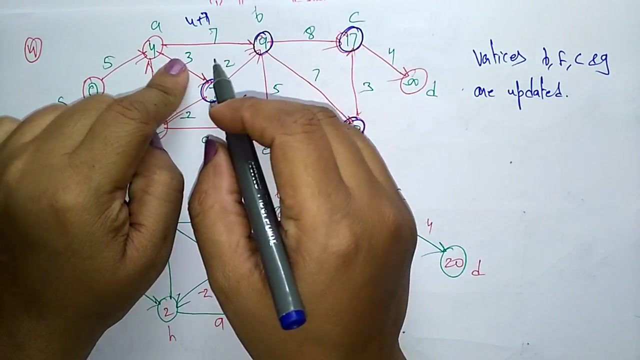 B, F, C and G has to be updated. What is this? B, F, C and G are updated. So with what values we have to be updated? So now check. So: from B, 4 plus 7.. 4 plus 7 is 9.. No, That is sorry. This is going from this. right, right, Okay. 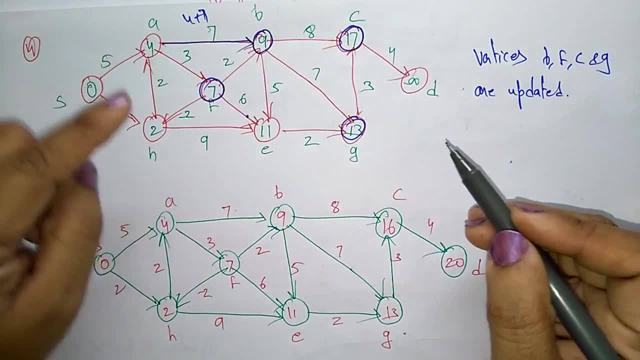 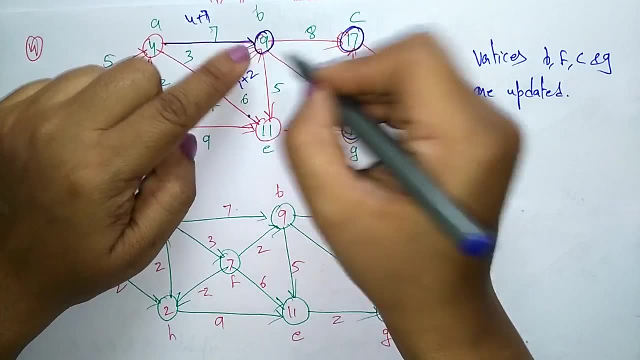 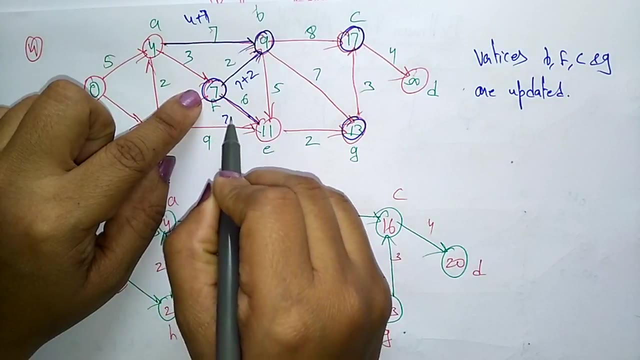 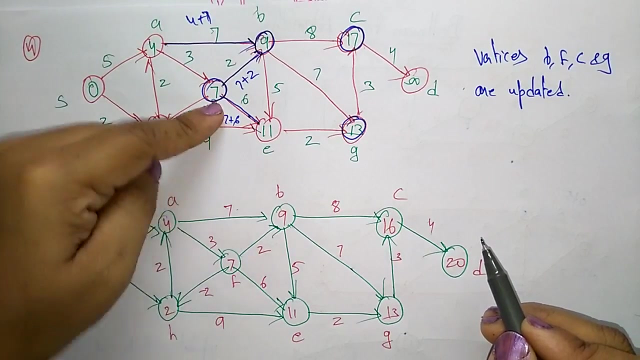 Okay, So, But 4 plus 7.. Now check here: 7 plus 2.. 7 plus 2 becomes 9.. Okay, This is satisfied. 7 plus 2, 9 is satisfied. Now check this side: 7 plus 6.. 7 plus 6.. So F. So this is not satisfied. 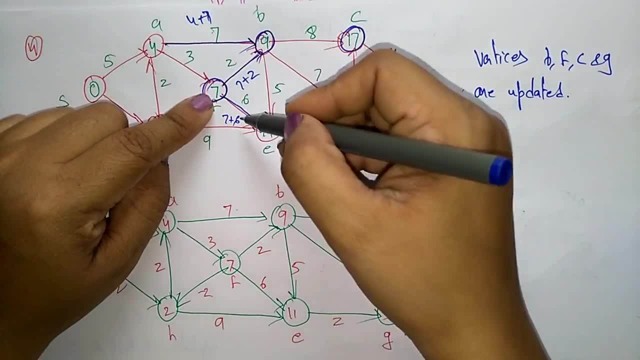 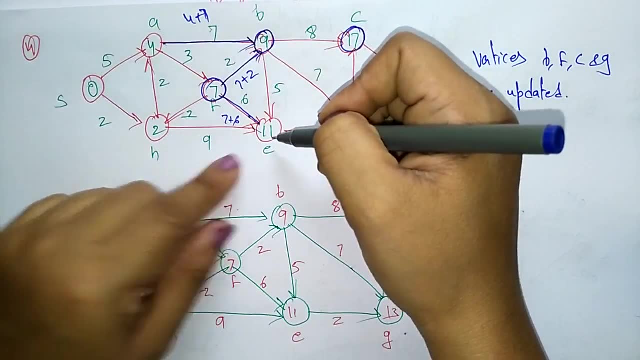 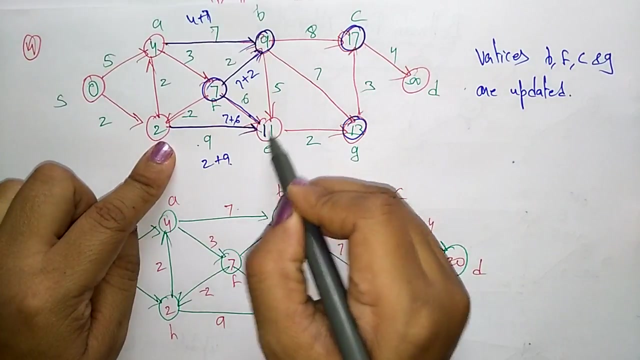 here: Okay. So 7 plus 6. It is not reaching 2. It's becoming 13.. So this is not satisfied. Now check here: 2 plus 9.. So 2 plus 9.. Okay, We get the 11.. So this, this path, is okay. Okay, So this is 0 plus. 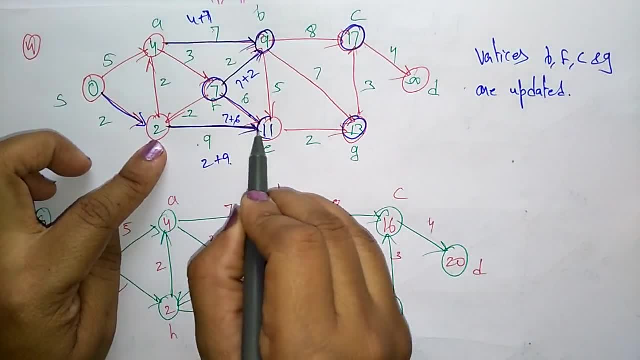 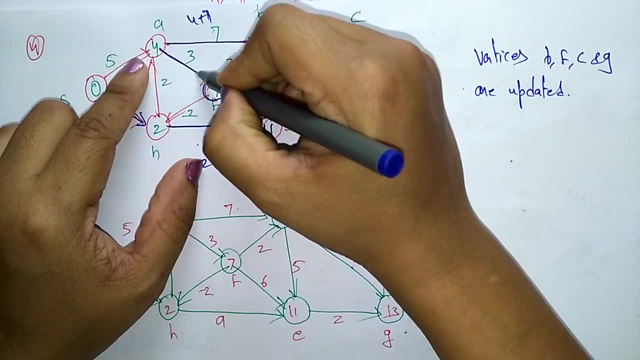 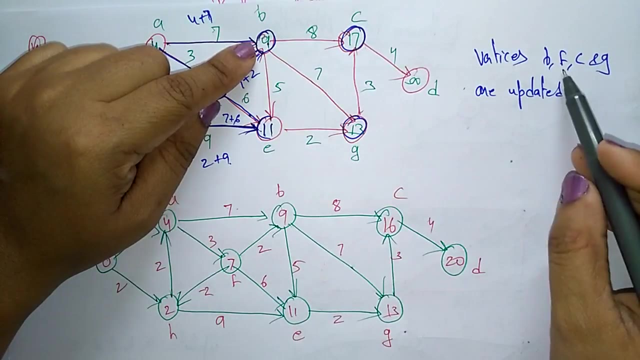 2 is okay And 2 plus 9 is okay. Okay, And coming to here, 7 plus 2 is 9.. Okay, And 4 plus 3. 7. This path is also okay. And now check here. I have to update C also: 9 plus 8.. 9 plus. 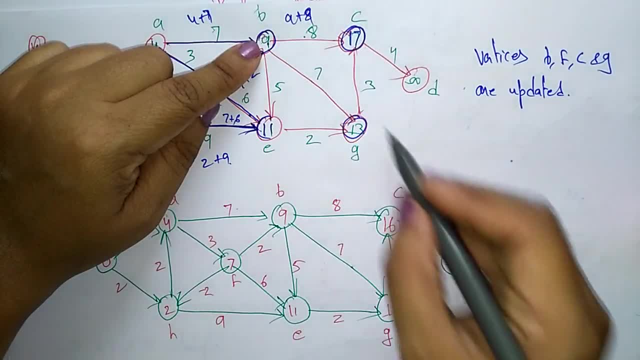 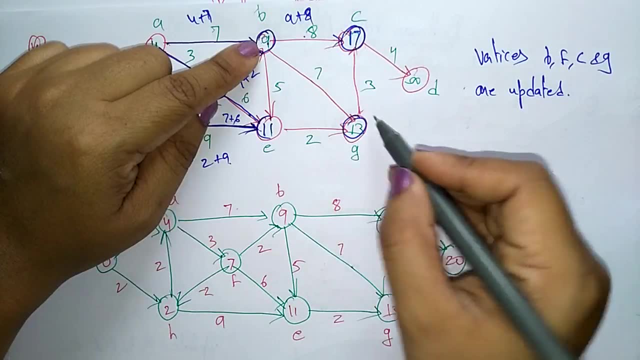 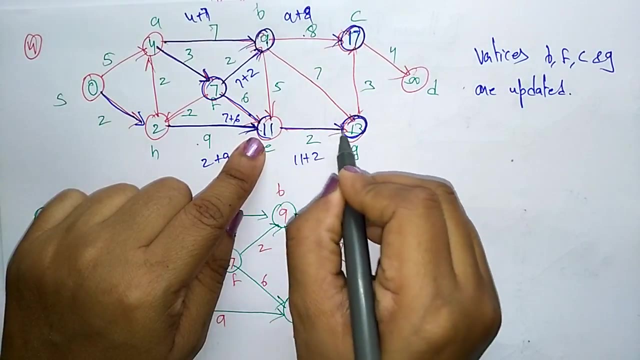 8. I'm getting 17.. Okay, This 9 plus. So first we have to check this. So this is a G, So G will come from 11 plus 2. This path 13.. So first, don't be confused. So first you. 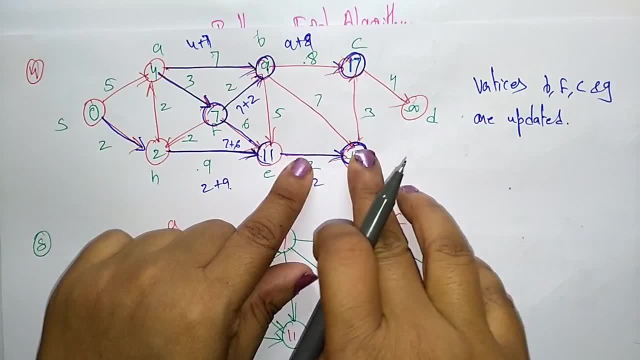 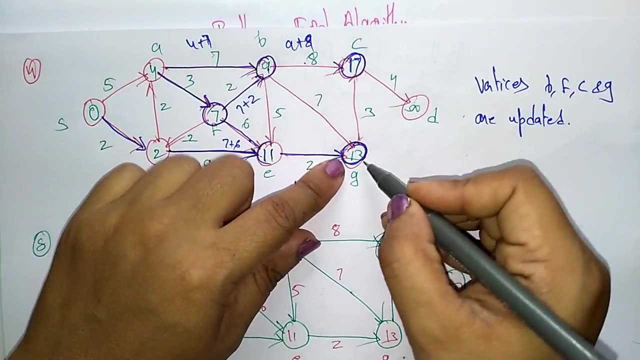 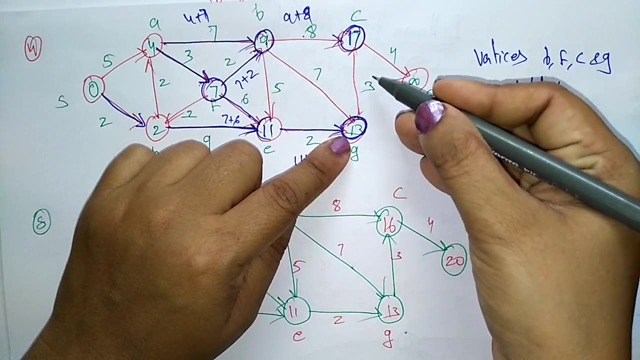 have to check one path Afterward. afterwards you check the other paths. If that path is not satisfying, you just discard that path. Okay. So here, 11 plus 2 is 13.. Okay, This is satisfied. Now I I'm checking this- 13 plus 3.. No, it's. you want the value it has. 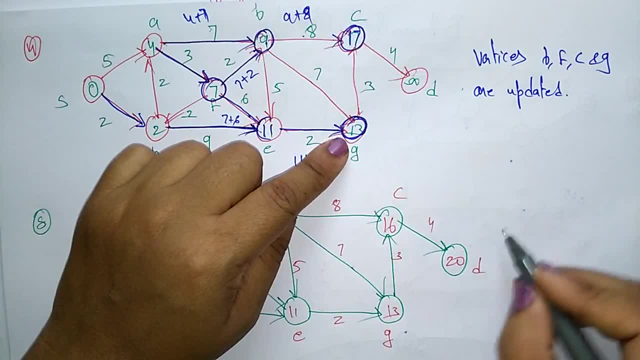 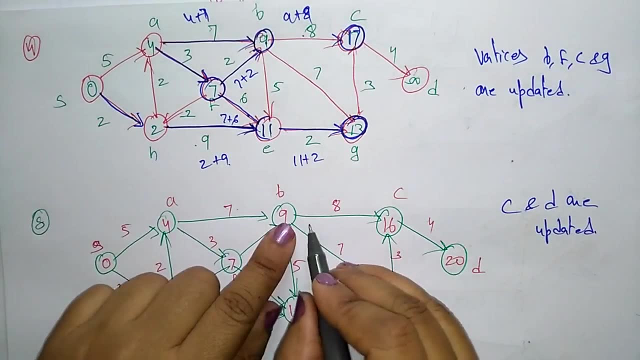 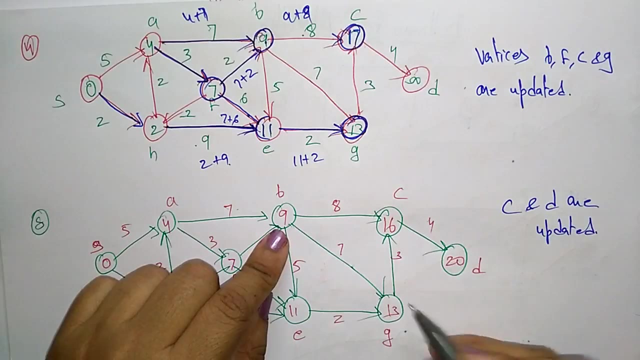 to be 16.. So now in the last, hence here the C and D vertices are updated with the new values. So now check here. So I mark it. whatever the value: 9 plus 8.. No, this 13 plus 3 is.